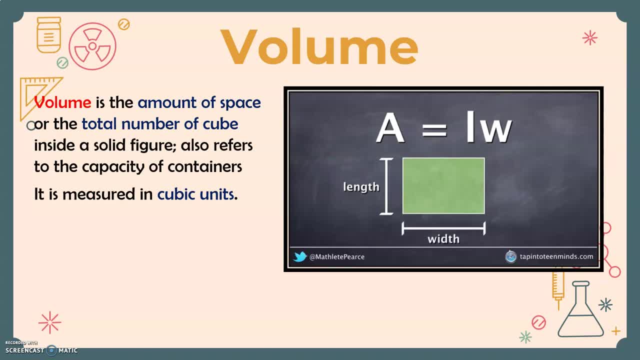 horizontal sides, which we will call our width. Let's put some numbers into this formula to give us a little bit of context. First, we'll begin with a length of 2, which means we're essentially going to be cutting this shape, this rectangle, in half horizontally, Because our length has a value. 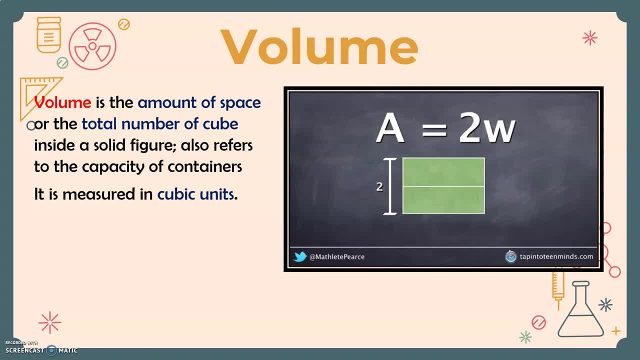 of 2. we're going to substitute 2 in for l in our formula. For our width, let's sub in a value of 3.. That means we're going to be cutting our shape vertically into three separate pieces. This also means we're going to be cutting our shape vertically into three separate pieces. This also means we're. 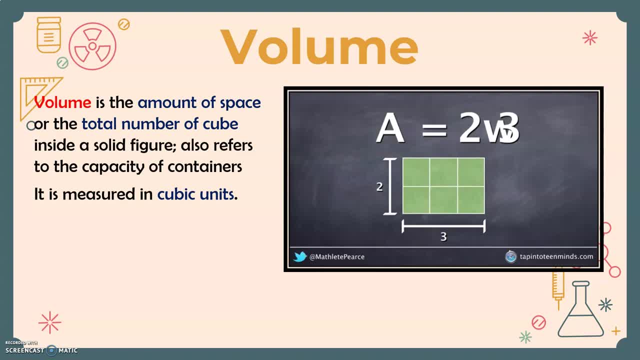 going to be substituting a value of 3 for the variable w in our area of a rectangle formula. By counting up the number of unit tiles in our 2 by 3 array in our diagram, or by multiplying 2 times 3 in our area formula, we can see that the area of this particular example is 6 units squared. 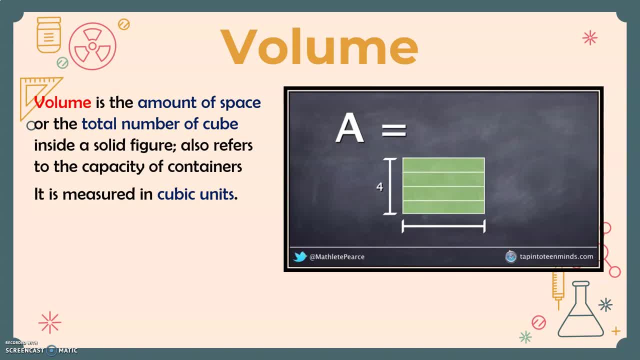 Taking a look at one more example. if our length is 4 and we divide horizontally the shape into 4 pieces and then look at a width of six, dividing the shape vertically by six pieces, we're going to get an area of 24 units squared. 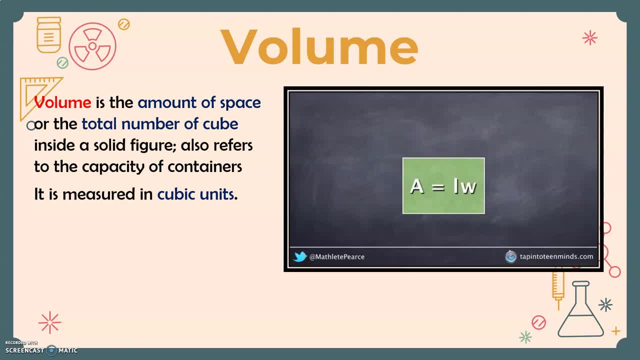 Now that we've looked at some examples for finding the area of the base, let's take a look at how this will relate to the volume of this rectangular prism, As we saw in the volume of a cylinder video. the area of the base is essentially the volume of this. 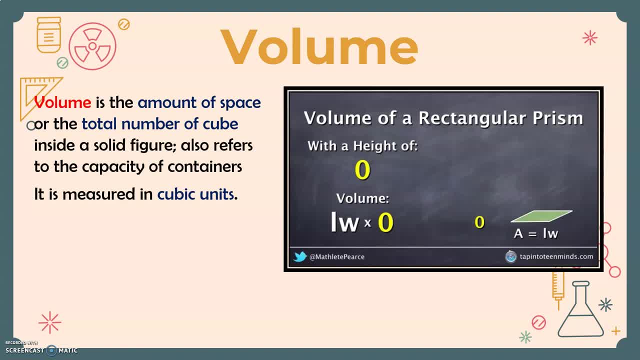 Prism with a height of 0. By increasing the height to 1 unit, we can see that we now have some volume to this Rectangular Prism. We can then increase this Rectangular Prism to a height of 2 by multiplying the area of a rectangle. 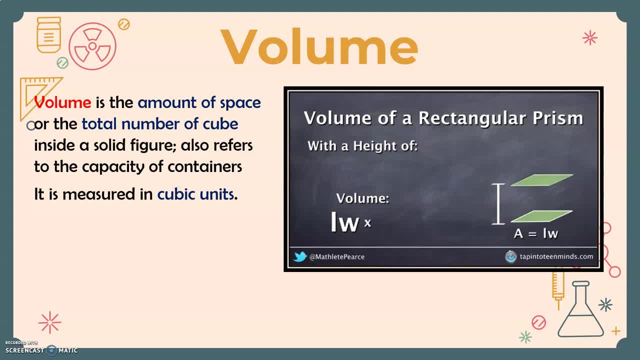 formula by 2, followed by increasing the height to any value by using a variable. In this case we're going to use the variable h- And thus the volume of a Rectangular Prism can be found by multiplying the area of its base times its height, or in other words, taking the length times the width of the base times. 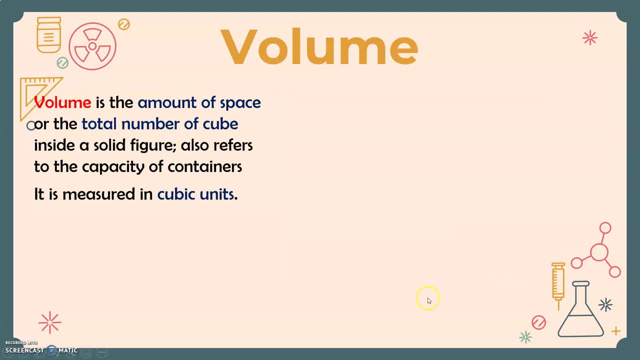 the height. Again, from the video we watched, volume is computed by simply finding the area of its base or the base of a rectangle, A solid figure multiplied by its height. So if we have a Rectangular Prism to find for its volume, we will use the formula length times width, times height. Now if 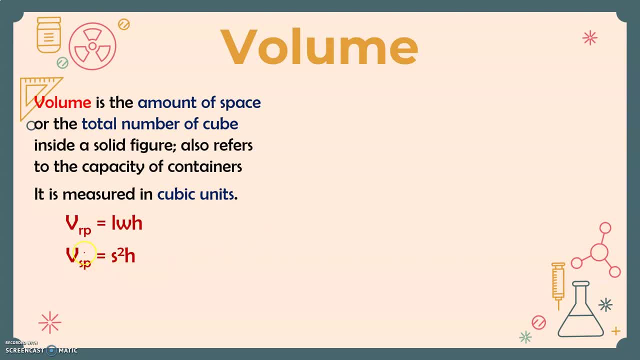 we have a Square Prism again to find. for its volume, we will get the area of its base times its height. That's why for our formula we'll have s squared times height. Now for the volume of a cube. we all know that in a cube 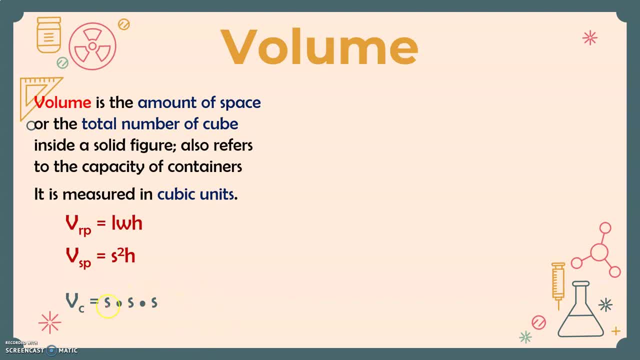 all its sides are equal right. So if you will find for the area of its base, that will just be side times side, and its height is just also equal to the measure of its height. So instead of using H here we'll just use s as well, because, again, 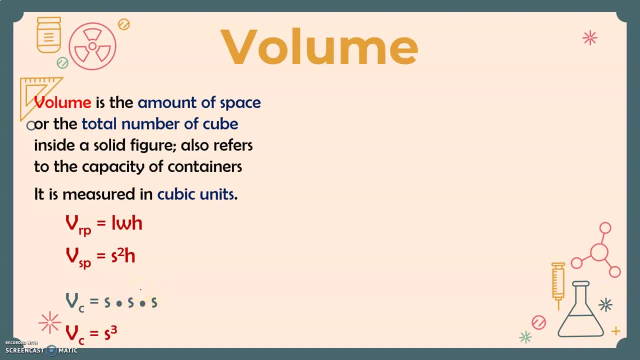 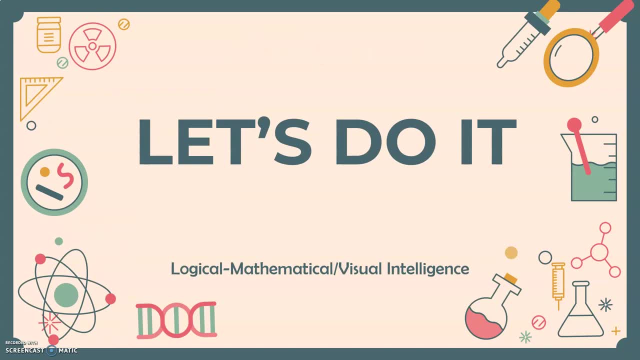 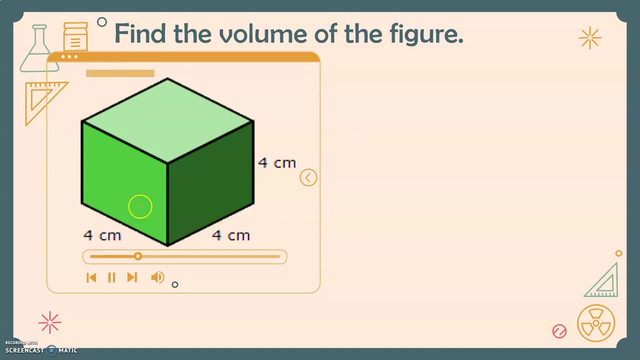 all sides of a cube are equal, So for its volume we can just simply use the formula s cubed. Let's try some examples. Find the volume of the figure below. So here we are given a cube, since the three dimensions given here are all equal, And for us to compute for the 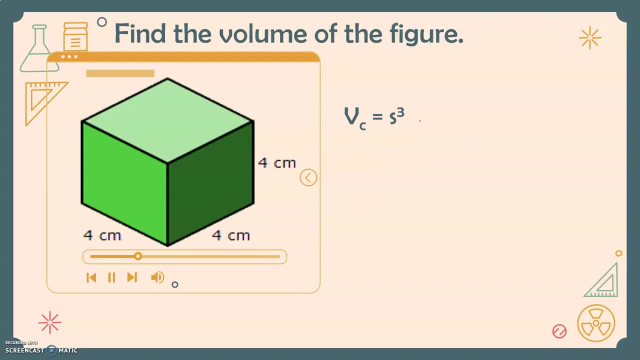 volume of a cube. we will use again the formula s cubed, Substituting the given information. we'll have 4 cm cubed. That means 4 cm times 4 cm times 4 cm and it's equal to 64 cubic centimeters. Again, volume is measured using cubic units, so we have here cubic. 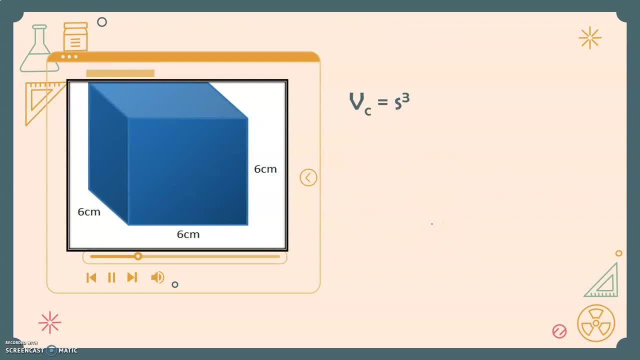 centimeters. Another one again. we are given a cube, so we will use the formula s cubed. Substituting the given dimension here, or measurement, which is 6 cm, we'll have volume of this cube equal 6 cm cubed, and that means 6 cm. 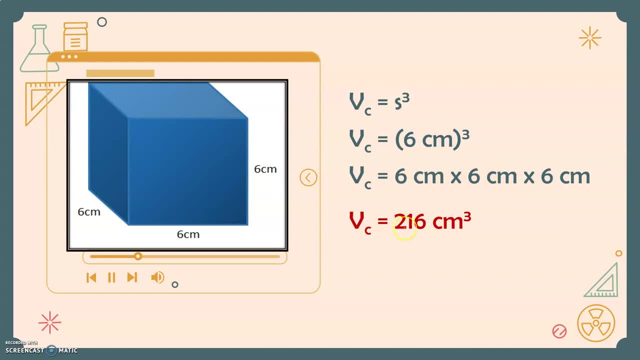 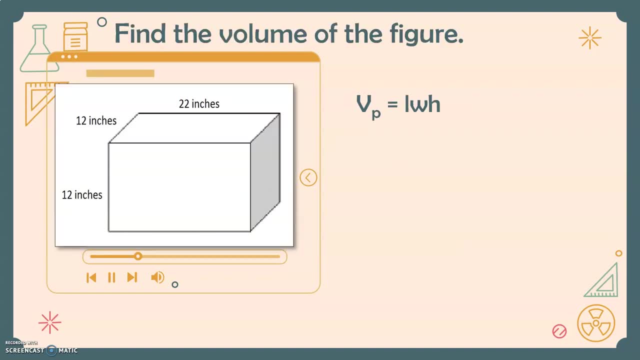 times 6 cm times 6 cm centimeters, which is equal to 216 cubic centimeters. Next, this time we are given a rectangular prism. So we have here a length of 22 inches, a width of 12 inches and the height of 12 inches. So for our formula we'll use length times width. 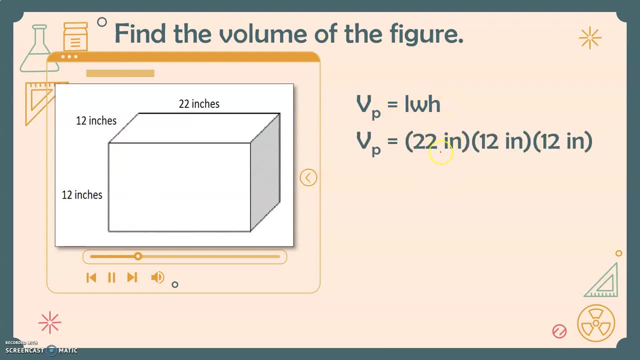 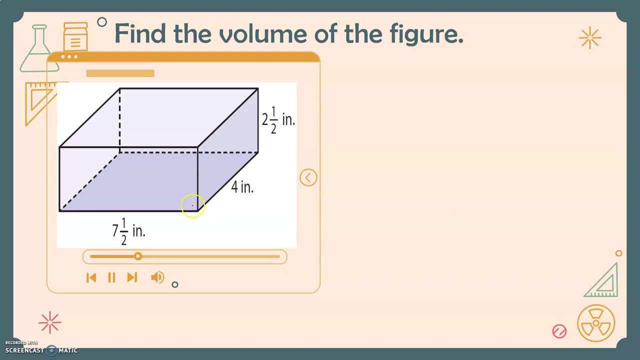 times height, Substituting the given information, we'll have 22 inches times 12 inches, times 12 inches, and that is equal to 3,168 cubic inches. Another example: Okay, this time we are given dimensions with fractions, But again this: 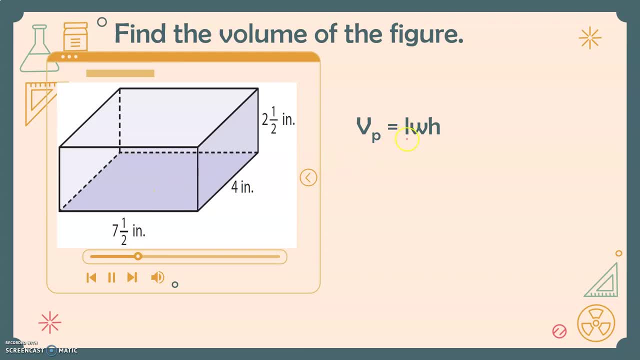 figure here is a rectangular prism, so the formula that we'll use is length times width times height For us to be able to compute for its volume. it will be much easier if we have a rectangular prism, So we'll use length times width. 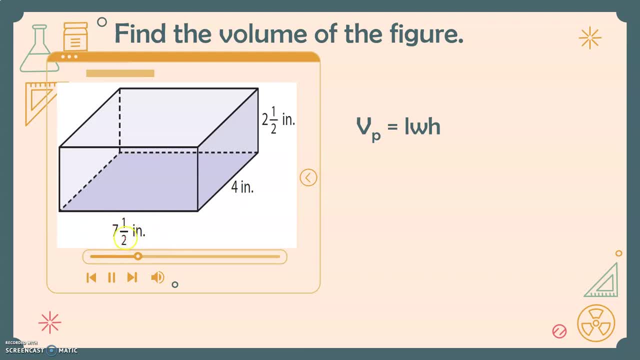 which is here for us to convert the fractions into decimal numbers. Since the fractions here are one-half, one-half is converted as 0.5 in decimals, So in our substitution we'll write 7.5 instead of seven and a half. Okay, so we have 7.5. 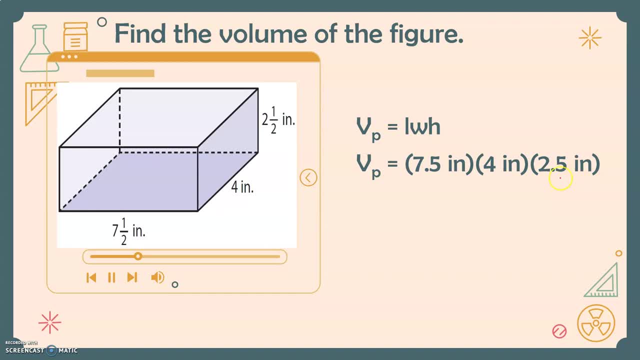 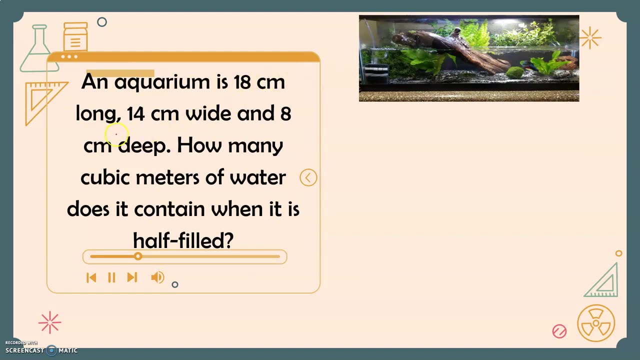 inches times 4 inches, times 2.5 inches, And that is about 1.675 cubic inches. Now let's try to solve this weird problem. An aquarium is 18 centimeters long, 14 zumindest wide and 8 centimeters deep. How many cubic? 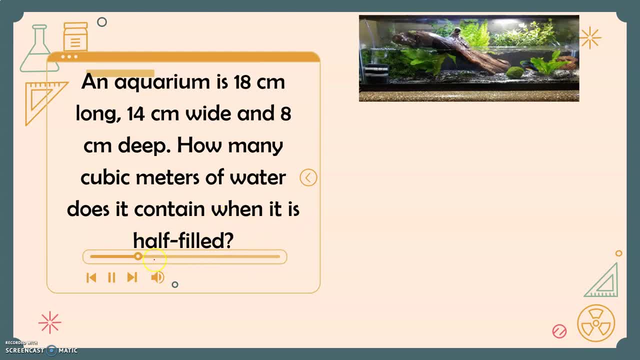 meters of water. this it contains when it is half filled. Okay, so we have here the keyword half filled. Now, since the aquarium is in the shape of a rectangular prism, we use the formula length times, width times, height. substituting the given information will have 18. 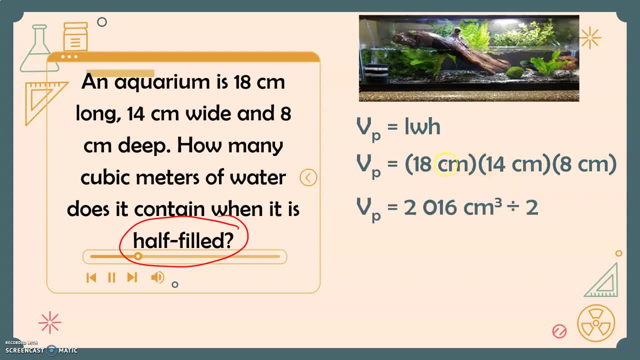 centimeters times 14 centimeters, times 8 centimeters, that is equal to 2016 cubic centimeters. but again, the question is asking for the water the the aquarium contains if it is only half filled, so we'll have to divide its volume by two.